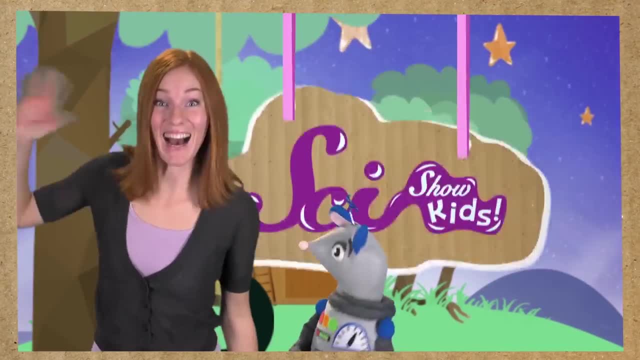 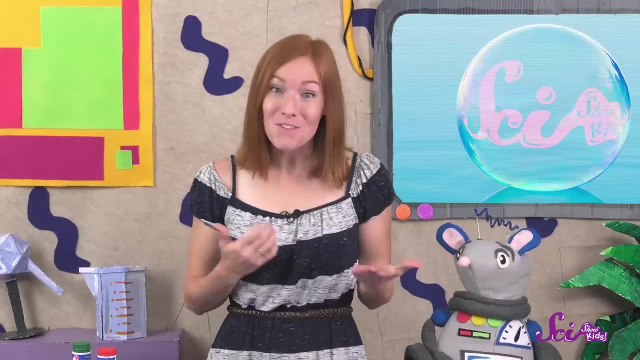 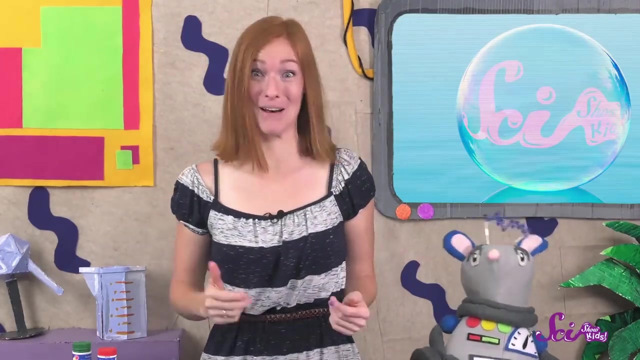 Today at the Fort we're blowing bubbles. This is an official summer fun alert. If you've had the chance to blow bubbles at school or in your backyard, then you know that it can be really fun to make them And to pop them. 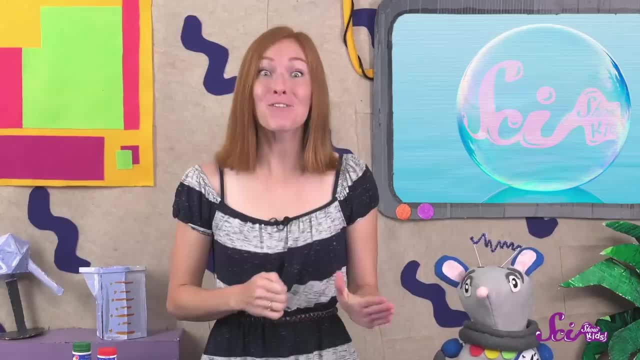 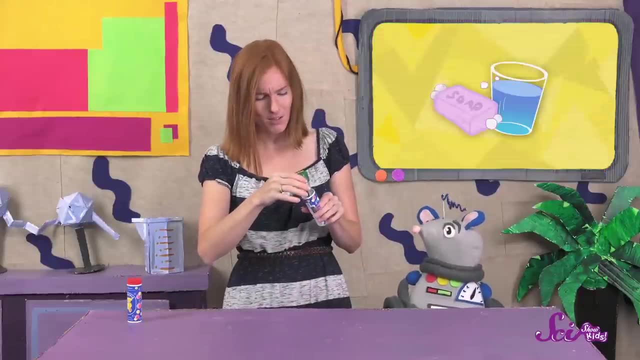 And they're also a pretty cool way to learn some science. First, let's practice blowing bubbles. To blow bubbles, you need two things: Bubble liquid, which is mostly made of soap and water, and the stick you blow the bubbles out of, which is called the wand. 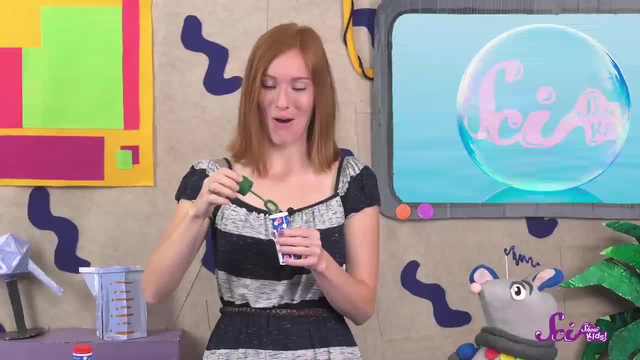 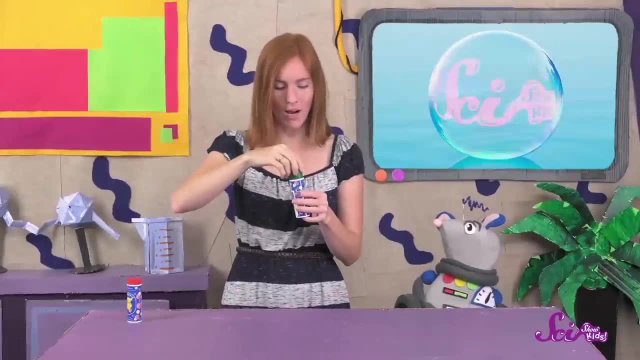 I'll dip my wand into the bubble liquid and blow, But not too hard. If I blow too hard then I'll blow the liquid right out of the wand. So I need to blow a steady stream of air through the bubble liquid. nice and slow. 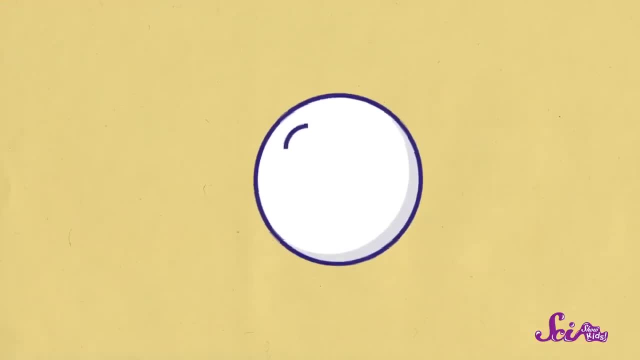 And I get a bunch of bubbles. Bubbles are just a really thin layer of soap and water around a pocket of air. If we could cut a bubble in half and look at it really closely, we'd be able to see the bubbles. If we could cut a bubble in half and look at it really closely. 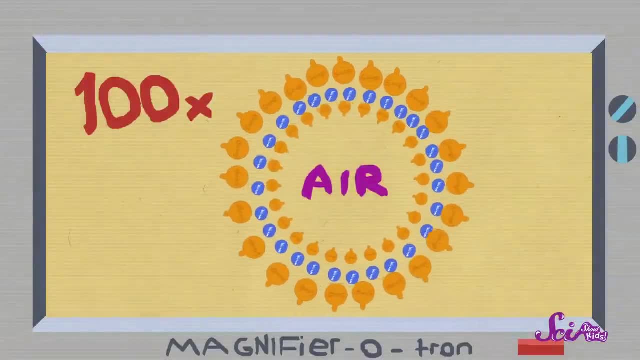 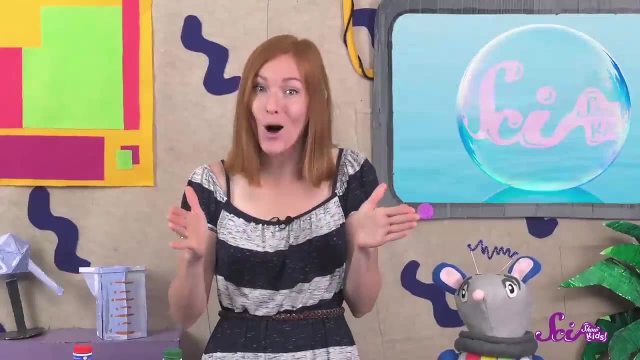 we would see that the bubble is actually made up of layers. There's a layer of water between two layers of soap. It kind of looks like a sandwich. The soap layers are like the bread of a sandwich and the water is like the sandwich filling. 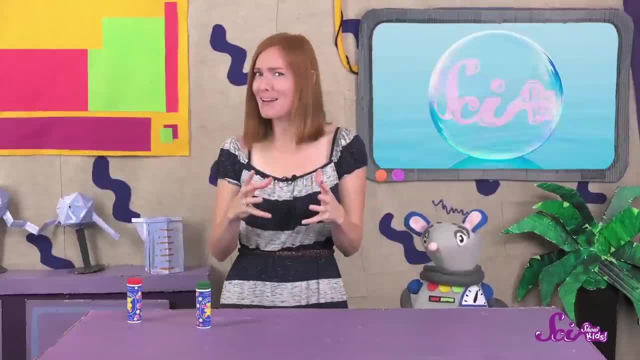 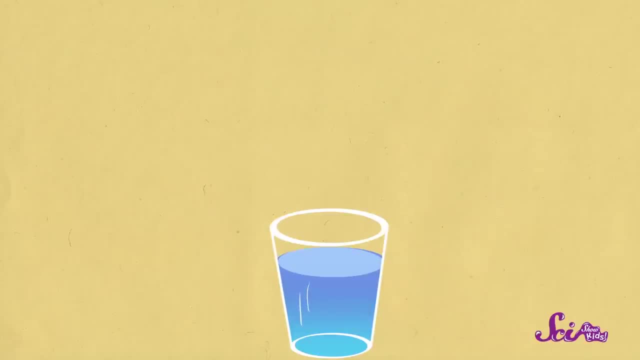 The layers of the bubble surround the air inside the bubble and keep it inside. Water without soap doesn't make bubbles very well, because water likes to stick together. Water's made up of lots of little tiny pieces or particles, so small that you can't even see them, but they're there. 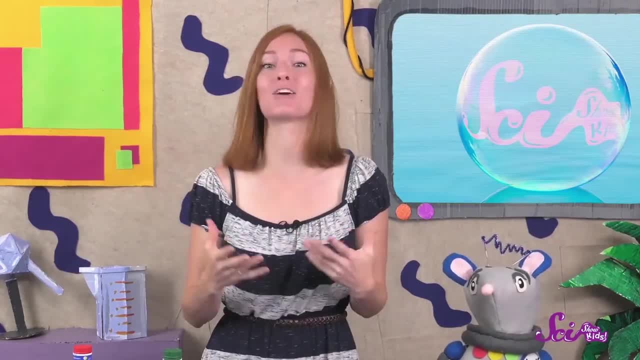 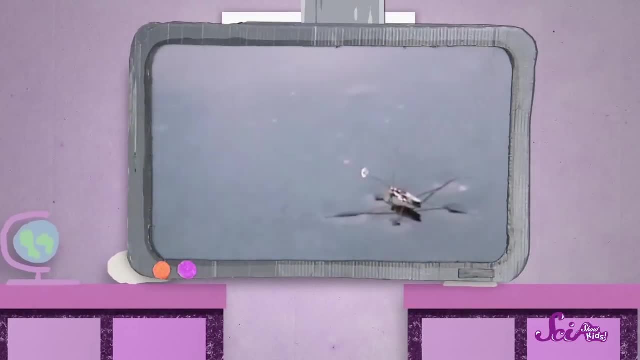 These particles are a lot more attracted to each other, meaning that they're pulling towards each other like magnets, so they stick together. For example, check out this insect. It can walk on top of this pond because the particles that make up the water in the pond 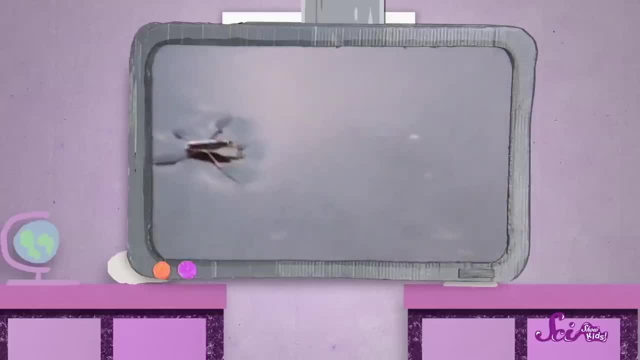 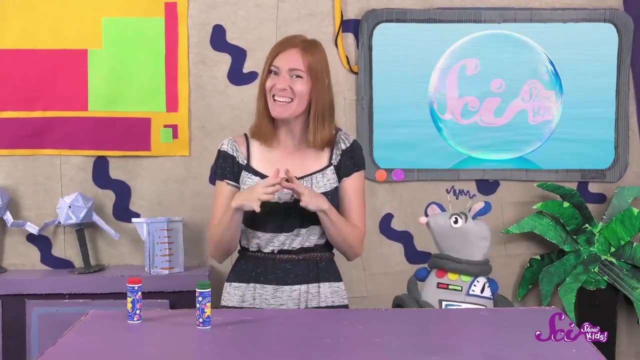 are all attracted to each other. They stick together so much that the insect can walk on the water without falling in. The little particles in water are pulled together so strongly that they can't spread out into a thin bubble with air inside. If we tried to blow a bubble with plain water. 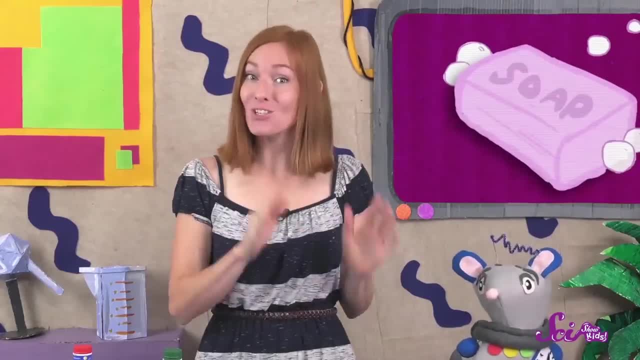 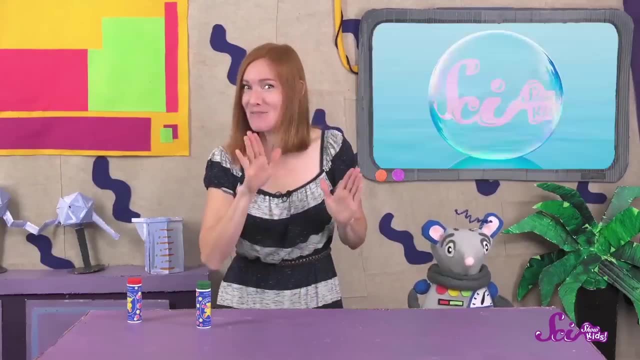 the bubble would just pull back together into a water droplet. But when you add soap, it helps the water spread out without being pulled back together, by making that soap and water sandwich, And then you get bubbles. There's something else special about bubbles too. 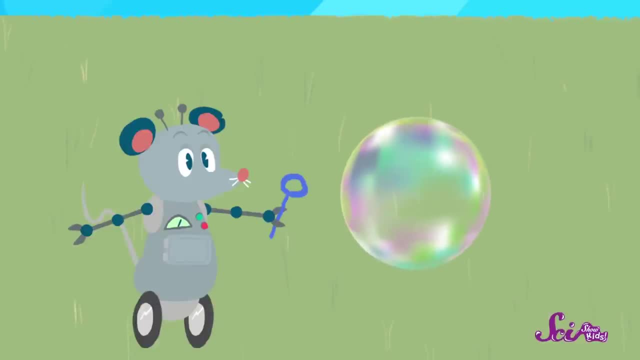 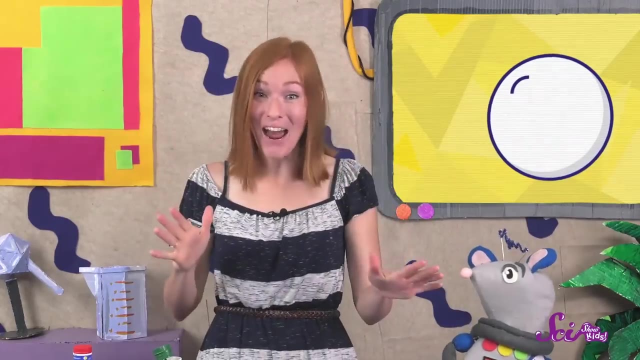 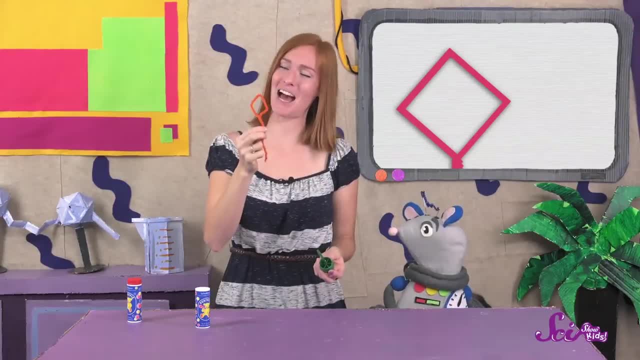 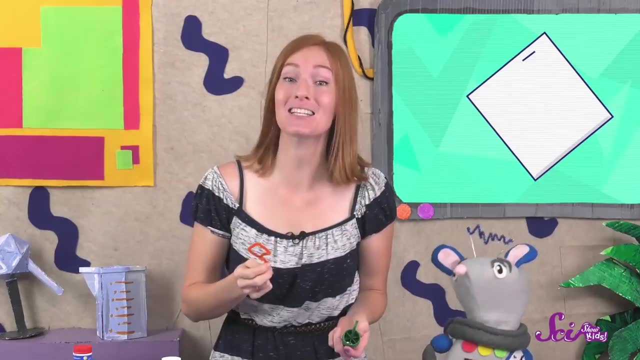 Like this one. That's right, It's shaped like a diamond. So what do you think will happen when I blow bubbles from this diamond-shaped wand? Squeaks thinks that they'll be diamond shaped. Let's try it and see what happens. 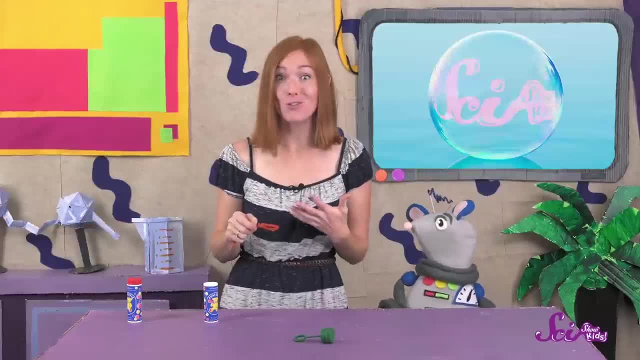 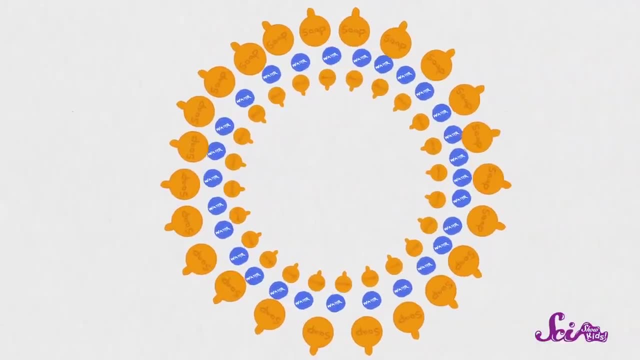 When I dip the wand into the bubble liquid and blow, the bubbles are still round, Even though the wand that I blew the bubbles from wasn't round. It's round because of that water layer, the filling of the bubble sandwich, Even though the soap helps the water spread out into a bubble by making the particles. 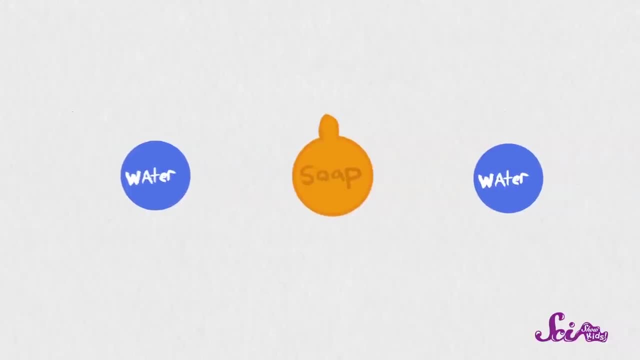 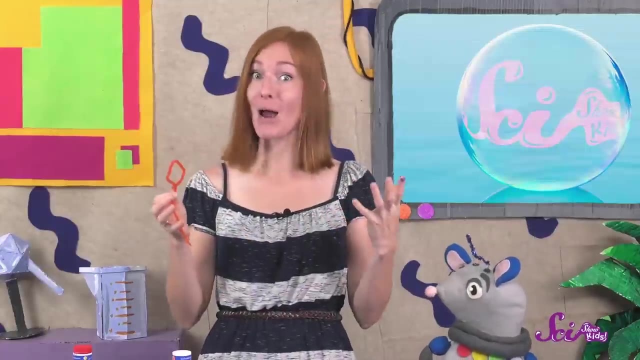 in the water less attracted to each other. they're still a little bit attracted to each other And when the water particles pull on each other around the air inside, they give the bubble its round shape. So even if our wand has corners, the attraction in the particles that make up water pull those. 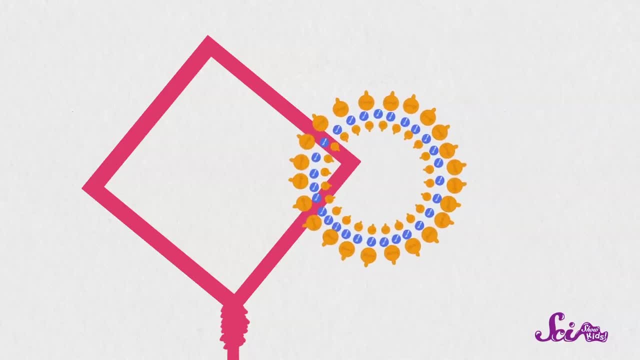 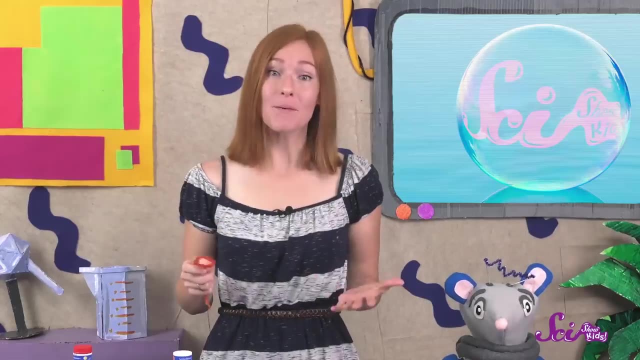 corners out and give us a nice round bubble every time. I guess you like popping them Squeaks Me too, But do you know why they pop If something breaks the attraction between the water particles that make up the bubble's? 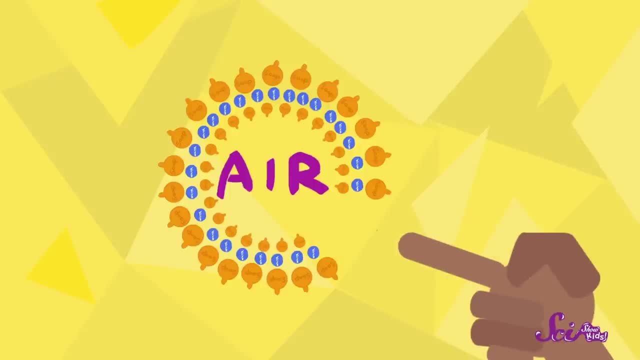 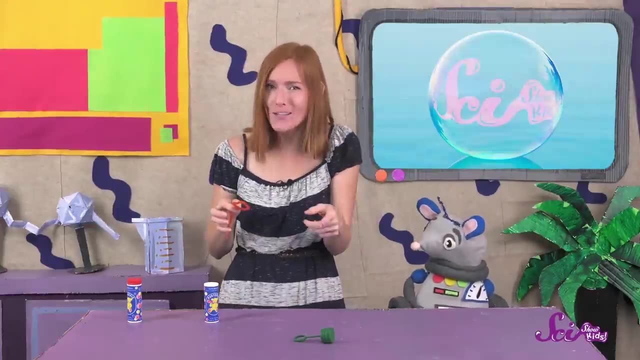 water layer, like Squeaks' nose or my fingertips. the air is able to get out and the bubble pops. It's a lot like popping a balloon with something sharp. When you poke a hole in the balloon, the air gets out and the balloon pops. 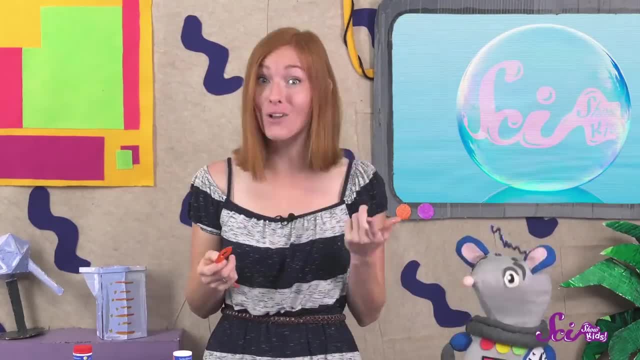 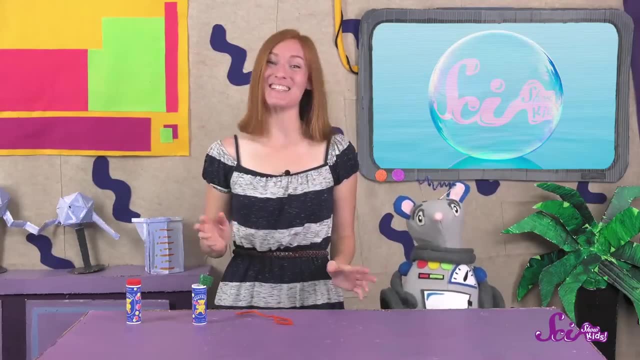 When you touch a bubble with your finger, you're basically poking a hole in the bubble. So do you want to pop some more? Okay, let's head outside and blow some more bubbles. Thanks for joining us. If you want to keep learning and having fun with Squeaks and me, hit the subscribe button. and we'll see you next time here at the fort.